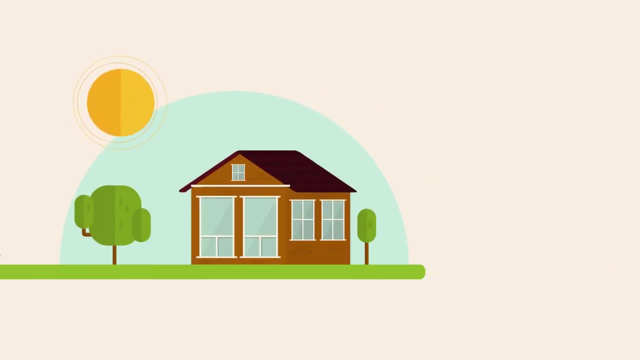 Well, you had to think of ways to reduce your use of fossil fuels. You might use energy to heat your home or cool it down, So put at least 40 cm of insulation made of mineral wool or similar in the attic. Have large windows facing the midday sun and small ones opposite. Fit triple glazing. 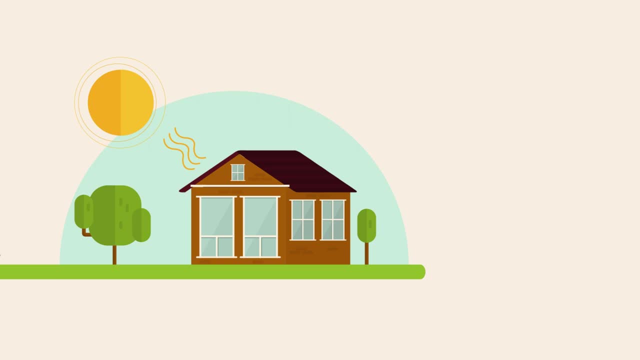 now standard for new homes in Canada and Scandinavia. Insulate the walls of your house well In hot climates, build verandas or have a central courtyard, as in ancient Rome or the Medinas of Morocco. With natural cooling, you avoid the need to use air conditioning or fans. 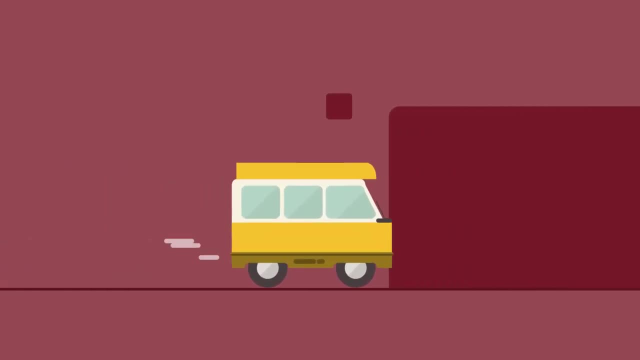 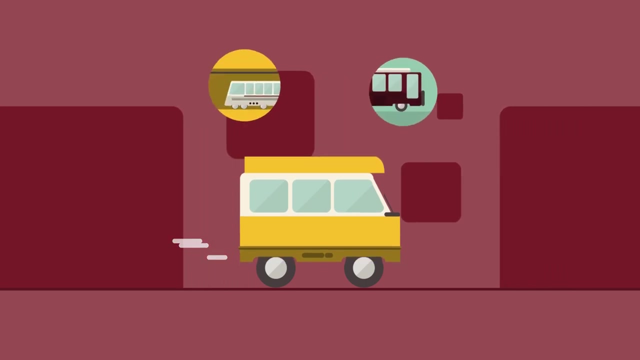 You might need to travel. If you have to use a car, reduce your speed. Most of the car's energy is used to push air out of the way. Better still, try to use buses and trains and, for short journeys, walk or cycle or take the bullet cart. 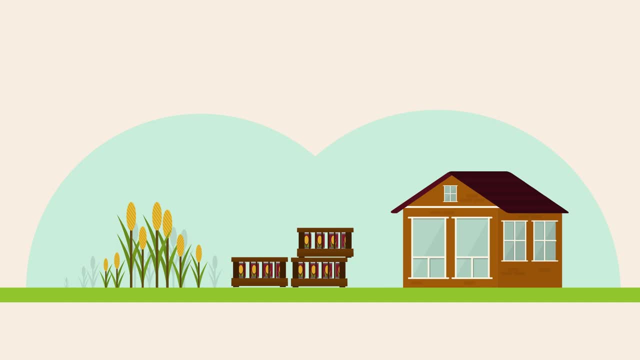 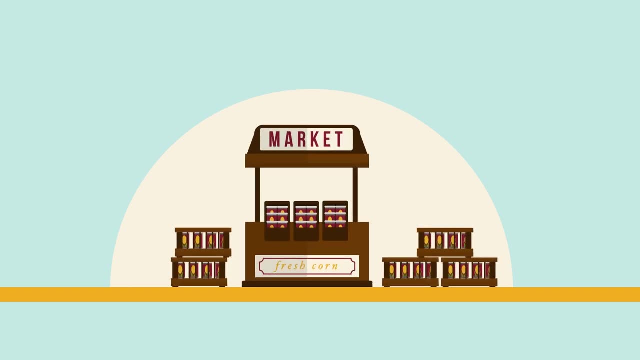 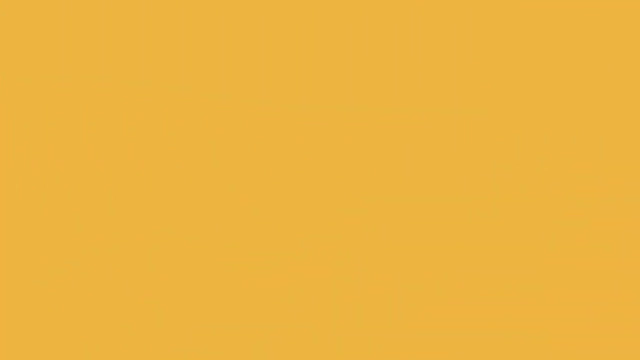 You need to eat, and growing and processing your food and bringing it to your house may have used fuel. If you cannot grow your own food, try to buy it locally to save transport costs. However, the main use of fossil fuels in agriculture is on the farm, For example. 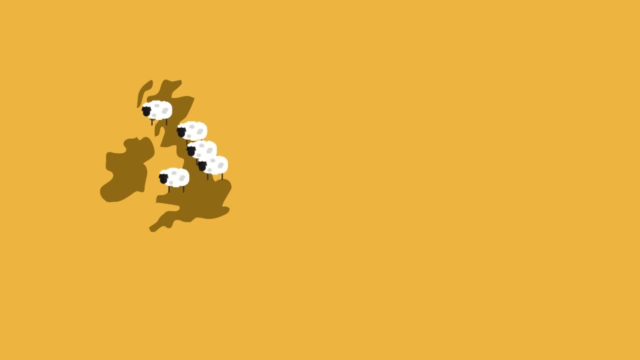 dairy and sheep meat production for the UK is more energy efficient if grown in New Zealand, even including the transport costs, because fertilizers are not needed in New Zealand, where sheep graze on hillsides unsuitable for human crops- Maybe the biggest way to reduce your carbon. 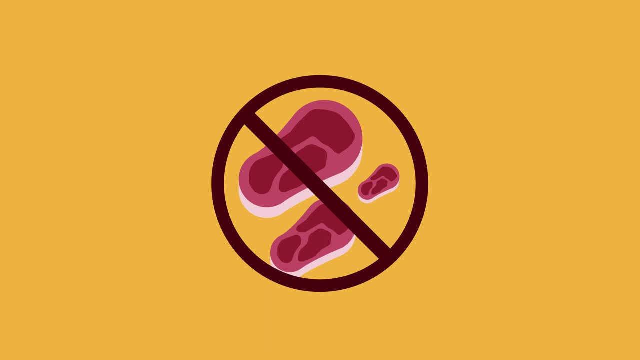 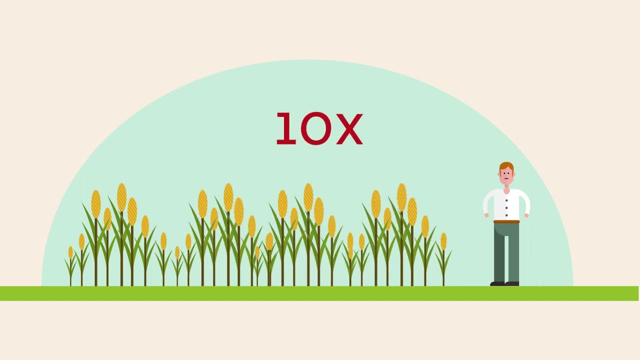 footprint is not to eat meat, especially red meat. By growing food for ourselves rather than for animals which we later eat, we can get up to 10 times as much food from the same land and fertilizer use. You may use electricity in the home. 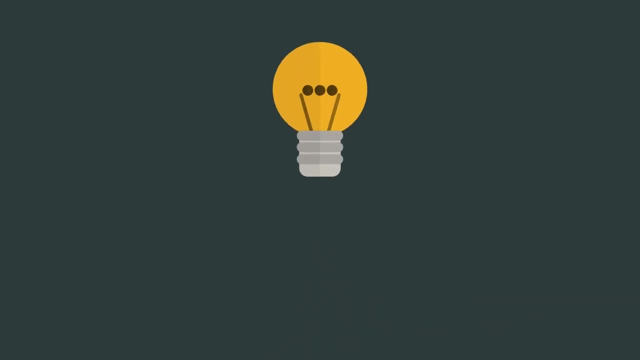 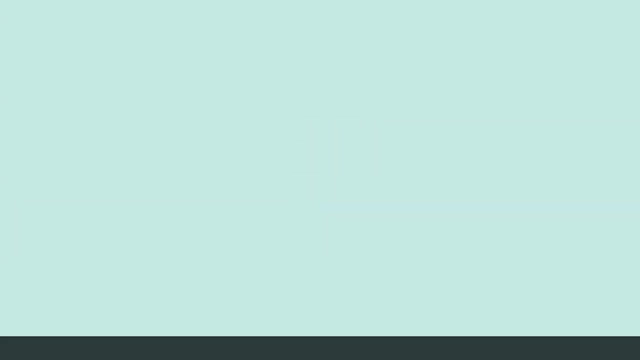 For example, what percentage of the electrical energy used by a filament light bulb comes out as useful light? Pause and think. Well, most of the energy comes out as waste heat and less than 3% as light. So replace your filament light bulbs with new LED lights which are nearly a hundred percent efficient If